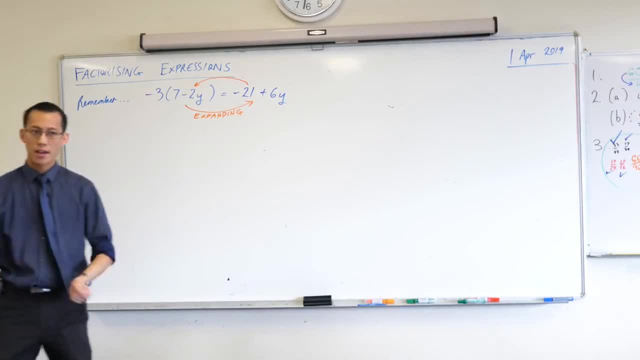 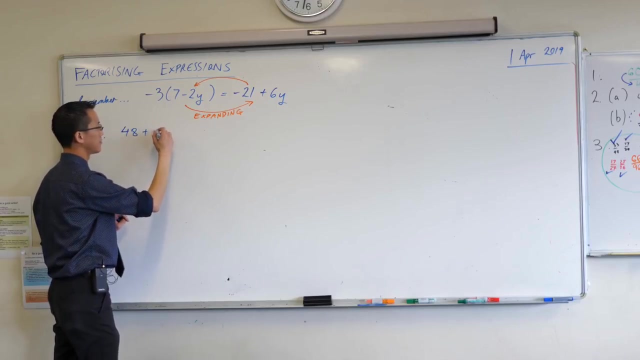 because that way, by the time I'm finished talking, you'll be ready Turn it on and boot it up. but let's think about some examples I think we can see here. I was just like: why is it not resolved? 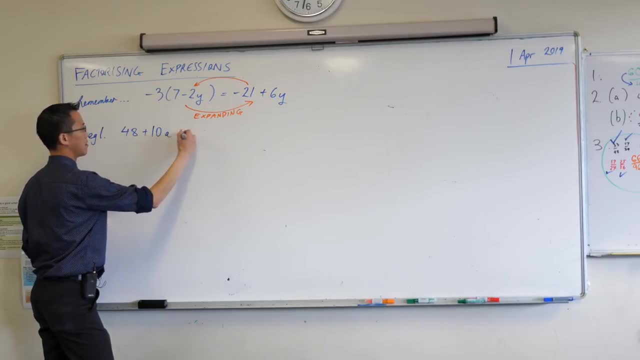 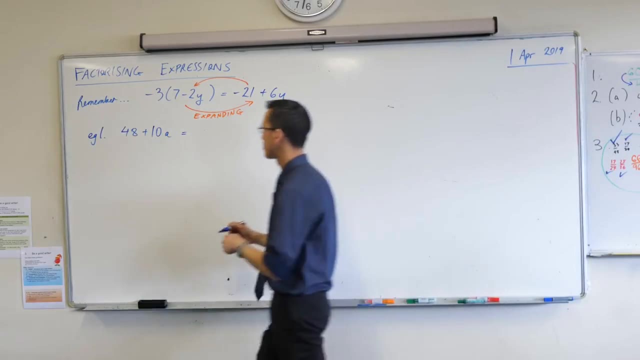 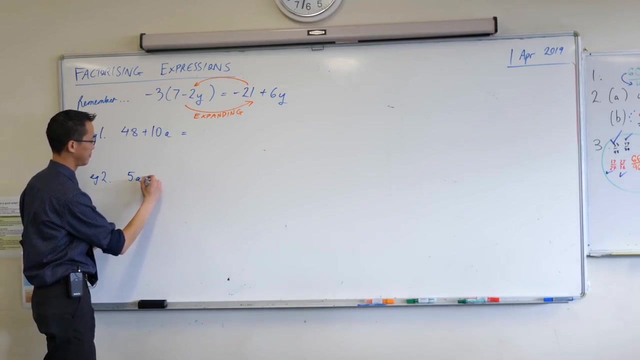 Okay, so here because I was just like genauing it, we don't do anything Right And hopefully a couple people are in here saying notes aren't in the book. But if you want to hear this yourself, the key is this is recursive right. 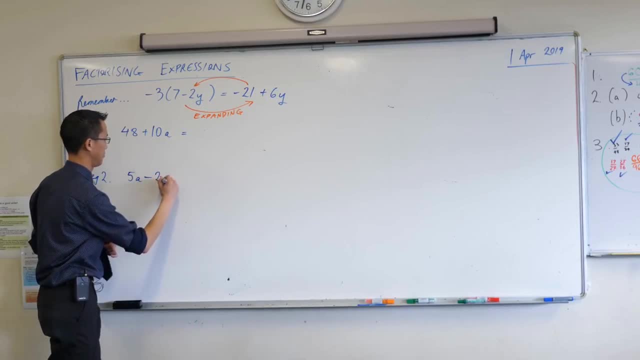 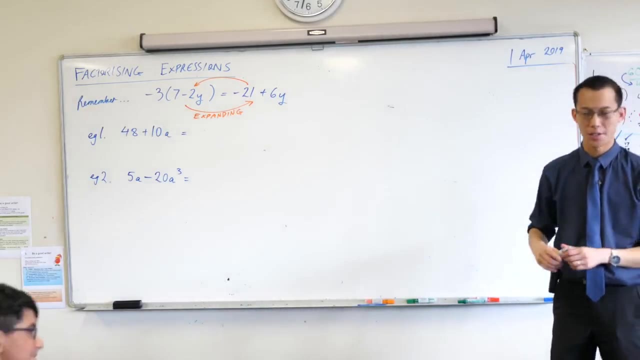 Maybe I'll just make myself go around the block a bit. You know, yelled back. we're really worried. there's 1973 written in it because I don't know if it would change at that point. We're factorizing all this. Okay, so your computer is opening up, but you don't need to speak, you don't need to look at it. I just want it to be booting up so it has time to prepare while working on this together. So underneath, where you've written that example of this is what expanding looks like. this is what factorizing looks like. 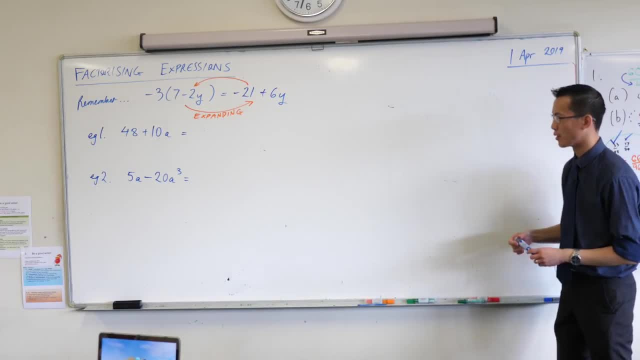 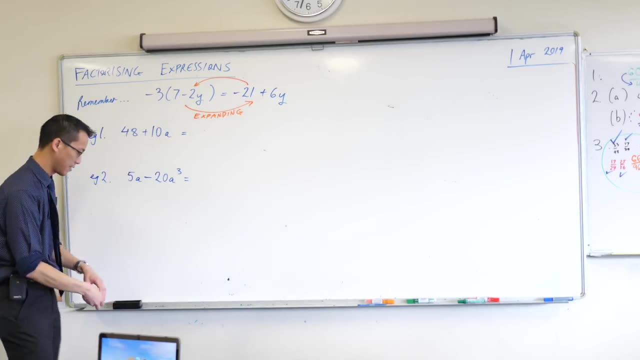 here's what it looks like when you haven't been shown before what it looks like. This is no brackets. we're going to factorize here. we're going to add some brackets in and, as the name suggests, factorizing. what you need to know is what are the common factors between the objects that you're trying to factorize? 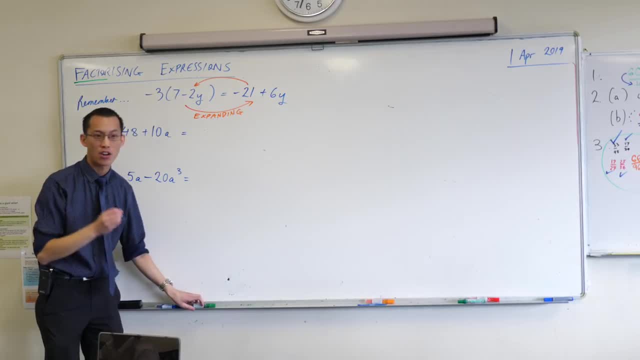 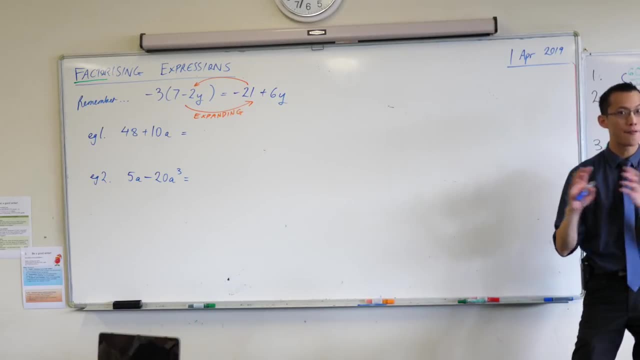 Okay, let me say that again. What you're searching for is a common factor between the two things you're trying to factorize. So this, hopefully, will remind you from last lesson. So when you think about 48.. And 10a, what's the biggest number that can factorize into both? 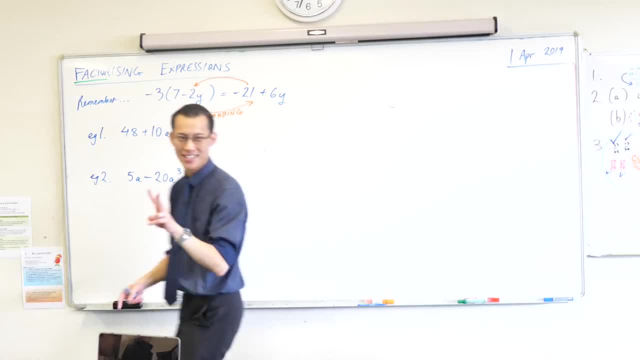 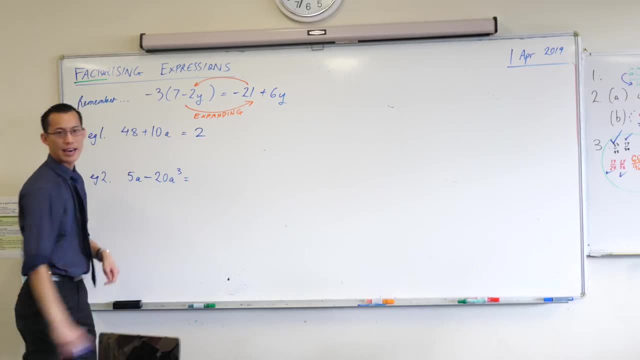 The biggest. yeah, It's just two in this case, isn't it? They're quite large numbers, but the biggest one that they actually share in common is just two, And one of the ways you can know that is, as soon as you write down, this factor out the front. 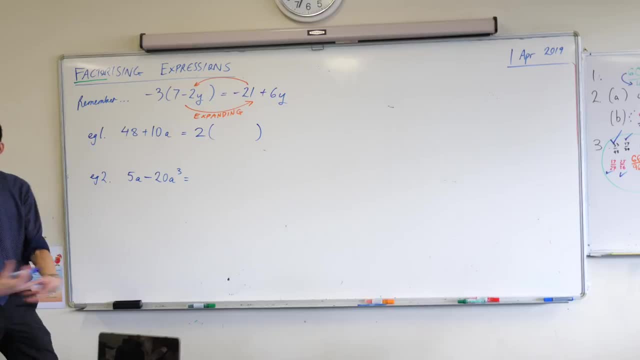 I'm going to write a pair of brackets- that's what factorizing introduces- and then I divide each of these by two. I'm kind of we call this- I'm going to take out a factor of two and put it out the front. 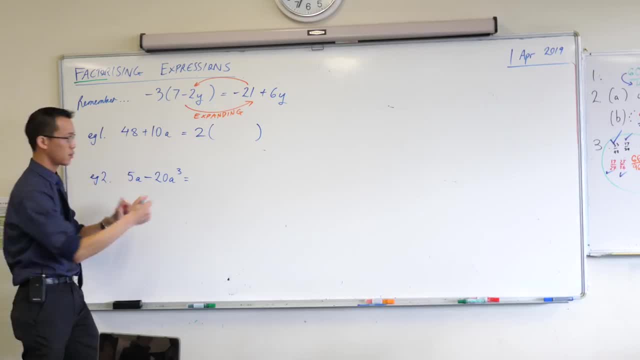 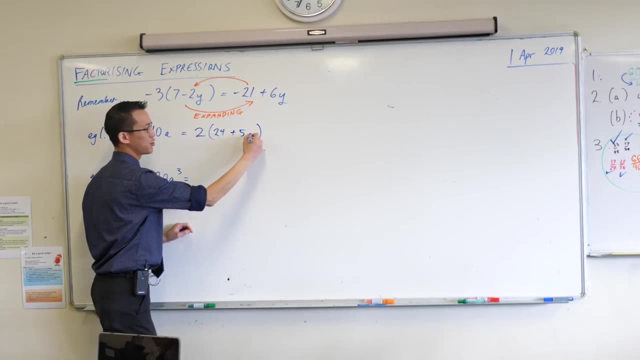 Okay, So when I divide this one by two, I get 24.. And when we divide 10a by two, I will get 5a. Very good, Now you can make sure that you can't have gone any further. you couldn't have picked any bigger numbers. 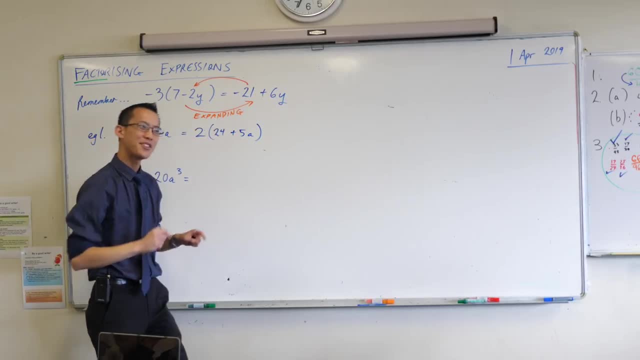 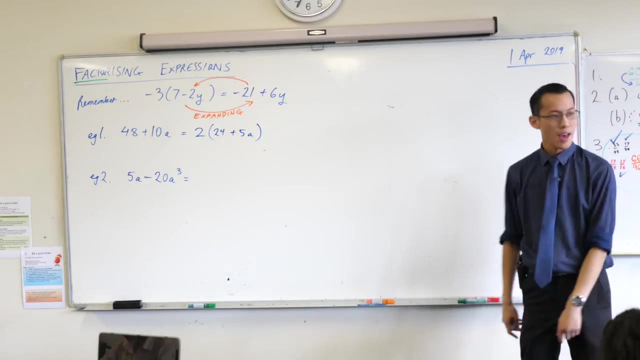 because you're like: oh, I don't see any common factors between these two except for one. but that's not very useful. Putting one out the front doesn't change anything. Okay, Now have a look at this next one. 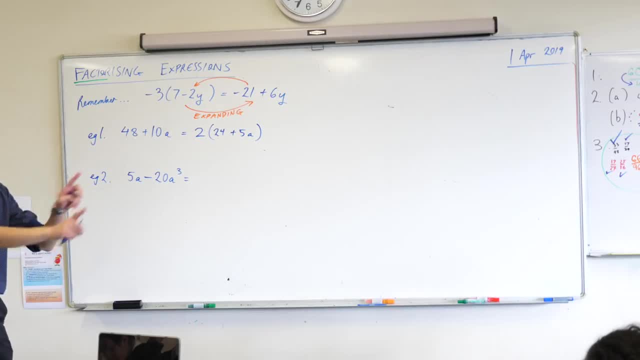 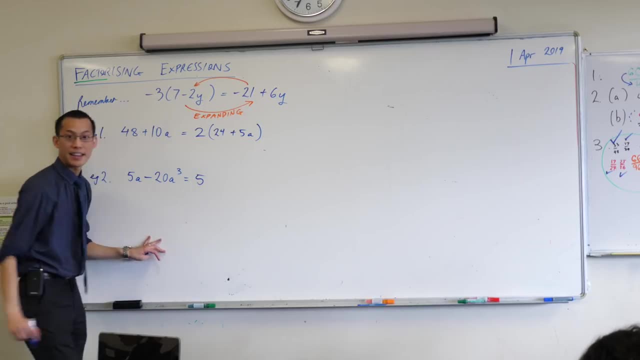 Okay, Now, for starters, let's just think about the numbers. We'll come to the pronumerals in a minute. Merrick, what's the biggest number that you see? Five, Five, very good, Now, first we'll write down that: five. 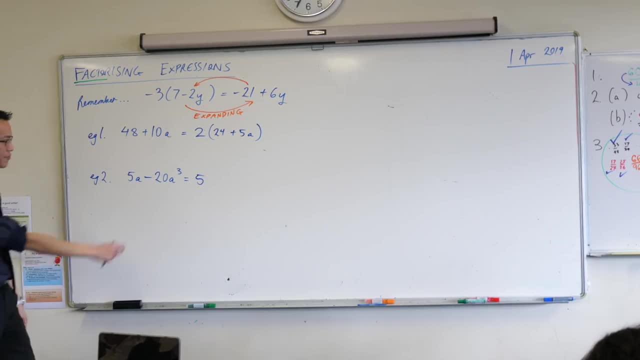 Okay, As you'll see in a second, there's going to be more work to do, but that's okay. I'm taking out a factor of five and I write my two brackets here and I divide each one by five. Now, Merrick, you just gave us the last answer, so let's see if we can get someone else to give us the next step. 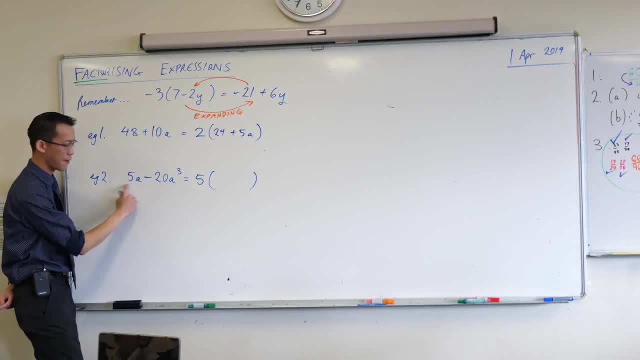 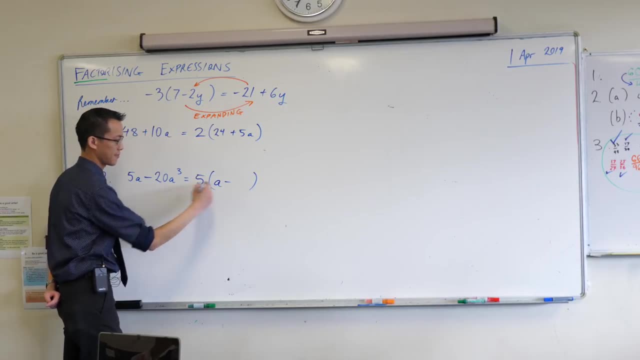 Okay. so, Henry, yeah, tell me what to do next. What happens when you divide this guy by five? Oh, I just did a. Okay, so Yes, And you can divide five by 20,, which is equal to four. 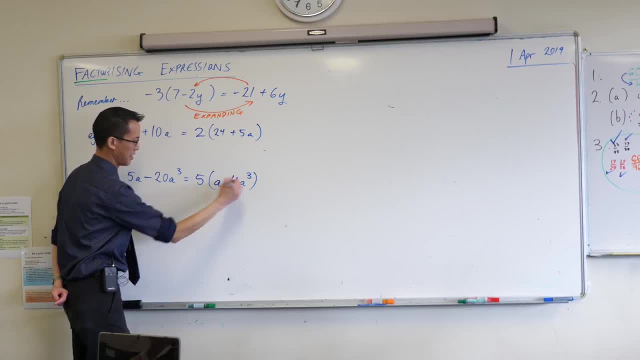 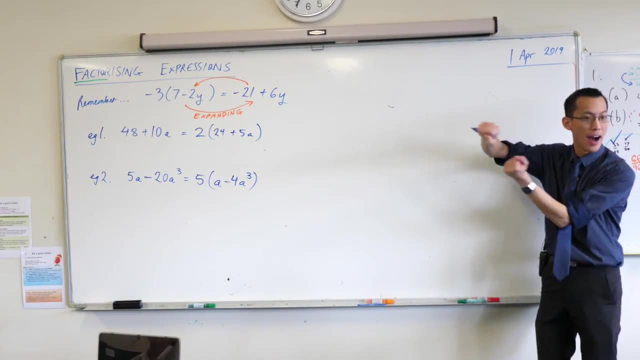 And then A by A is squared. Now, yeah, yeah, we're going to get to that in the next line, right Now. what have we done here? We took out a factor of five, so I've divided everything on this side by five, and that gave me what's inside the brackets. 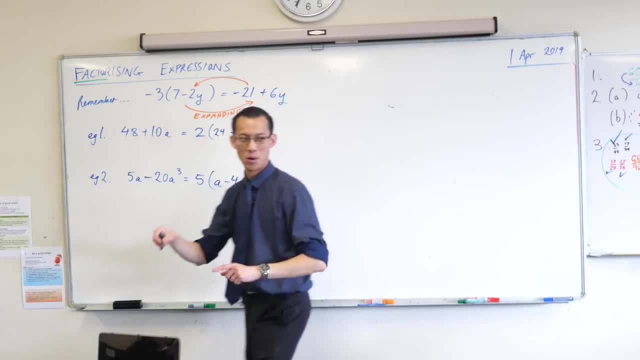 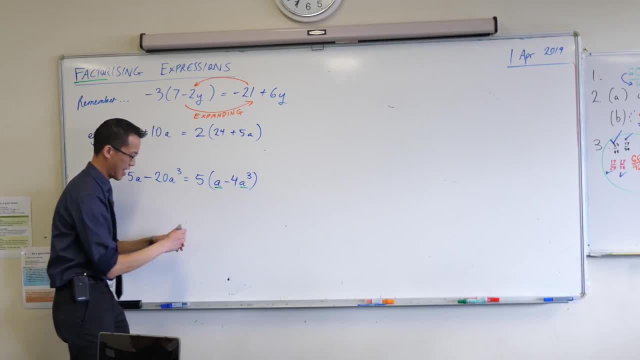 But in this case, unlike the previous one, I can do more, Jessica. what do you say? So then there's A and A cubed If you take the A out next to the five. Okay, so just pause that for a second, Jessica. 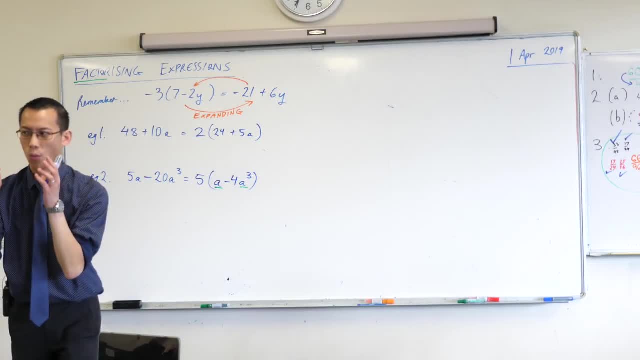 Hold that thought. Think about what we're doing here. right, We're trying to find the biggest factors we can take out. We took five. That is the biggest number, But A is also a number, isn't it? It's a perineum rule. 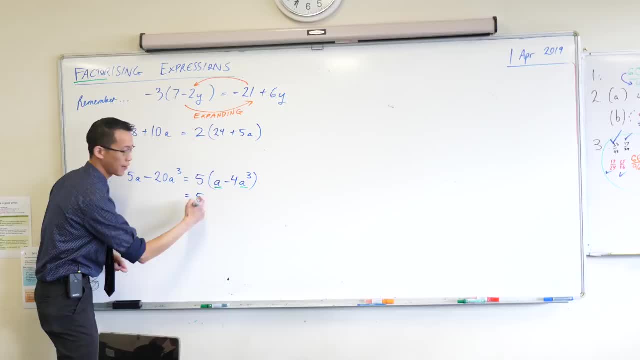 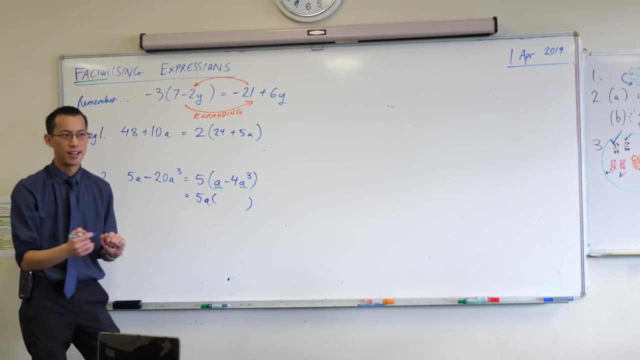 I just don't know what the number is. okay, So I can take out five. I've already done that. I can also take out this A that Jessica is suggesting, And then I'll have something even simpler left in here. Okay, Louise, do you want to tell me what to write next? 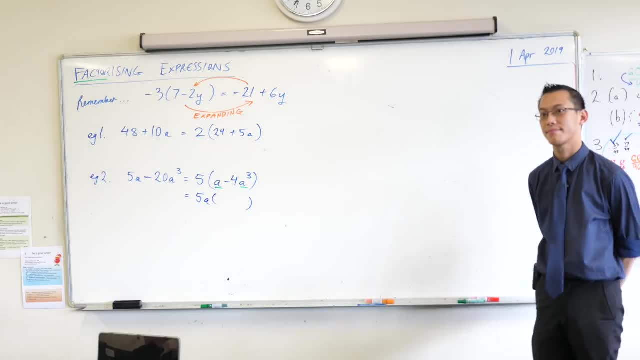 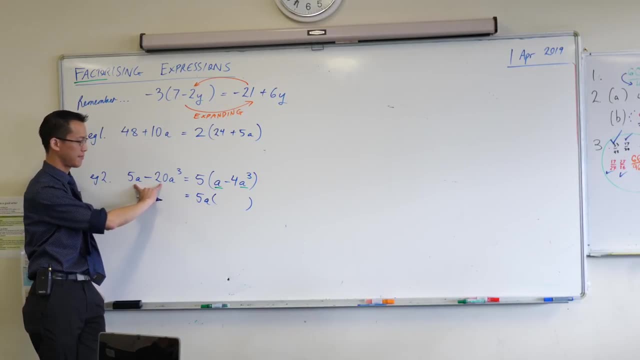 Oh yeah, go ahead. What do you want to ask? So how does it come that in 5A- like in 5 and 20, the highest common factor is five? Yep, And you can write five, but in the example one, 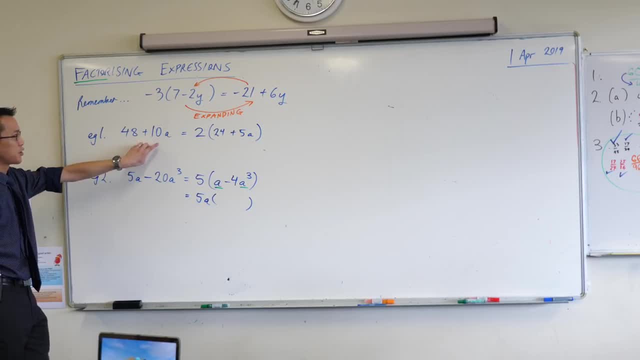 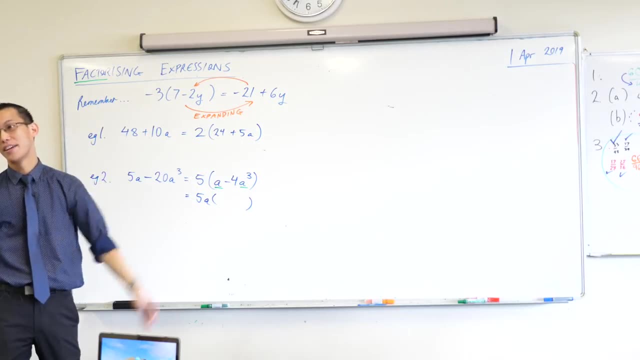 you write two instead of one. So why did I write two here? Is that the question? Yeah, Yeah, okay, It's always about the biggest number I can find, right. Let's think about this, right, If I had written down, I'm just going to write it in another color. 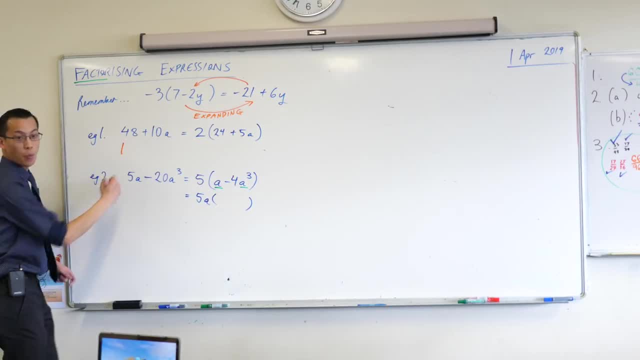 You don't need to write this down. If I looked at the first line, I'd say: oh, I can take out one. I'm going to do the same thing I've been doing every other time. right, I'm going to divide this by one, which gives me 48.. 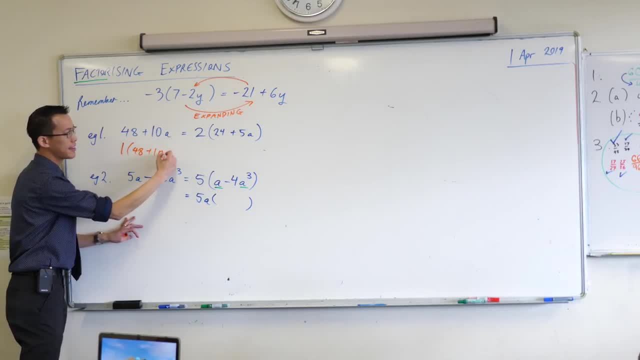 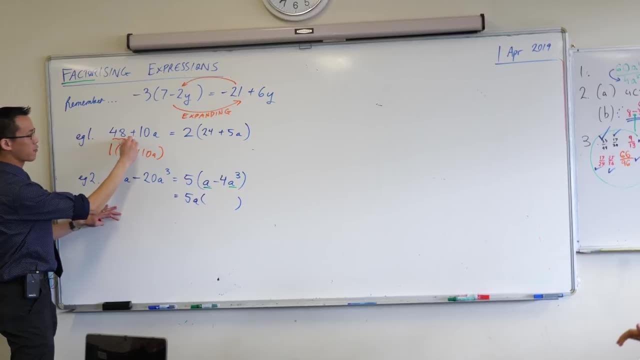 And then I'm going to divide this by one which gives me 10A. Now, this is a true statement. It's true. It just isn't very useful because it's kind of like, but I already knew that. That hasn't changed what I've got here anymore. 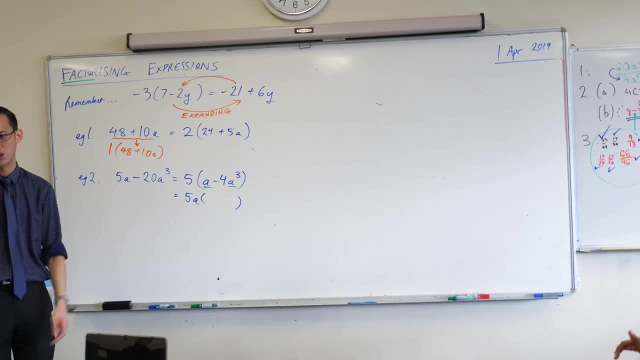 It hasn't made it simpler. Does that make sense? So you can do it. It just doesn't lead you anywhere, Krishan, For the member thing. so you do 3 minus 3 times 7, which would be minus 21.. 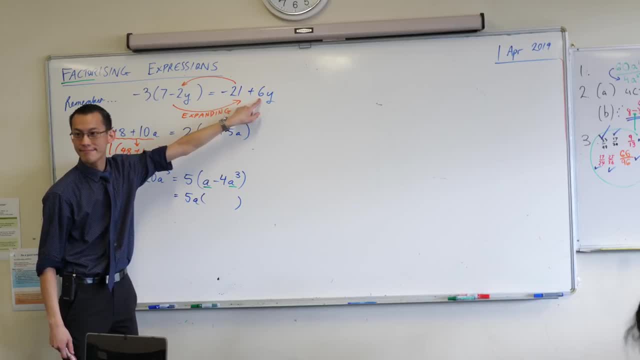 Yes, But to get 6Y if it's minus 3, how do you times it in positive? Okay, we're going to get to the negatives in the next one, if that's okay, because they are a bit sneaky and tricky. 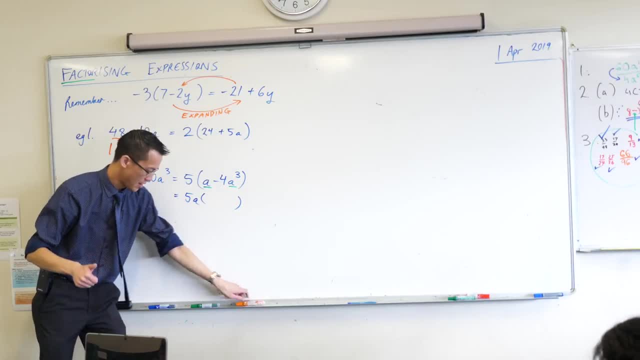 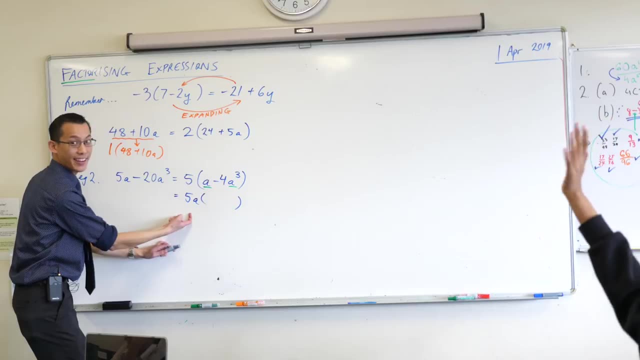 I've deliberately been giving you mostly positives. We'll have a look at the next one. okay, Is that all right? Now we're not quite done here, right? Can someone help me out? I'm looking at these guys. I'm dividing each one by A. 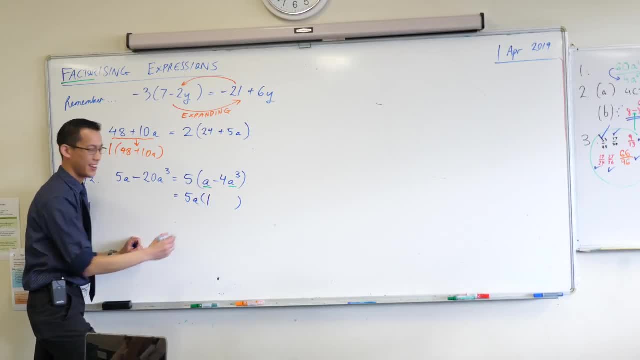 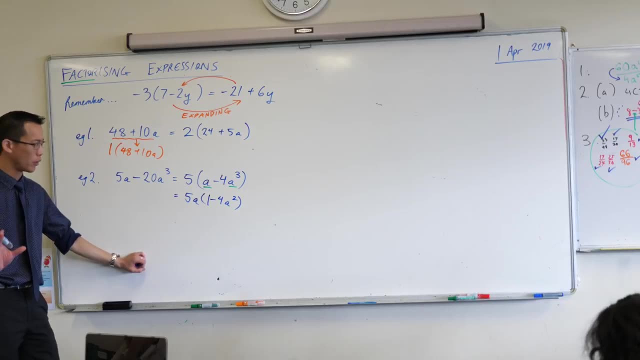 Okay, Jessica, give me what you've got. One Minus 4 is A squared. Just have a look at that with me, because that was a bit weird and different. okay, Boys, are you still with me? Thank you, everybody. 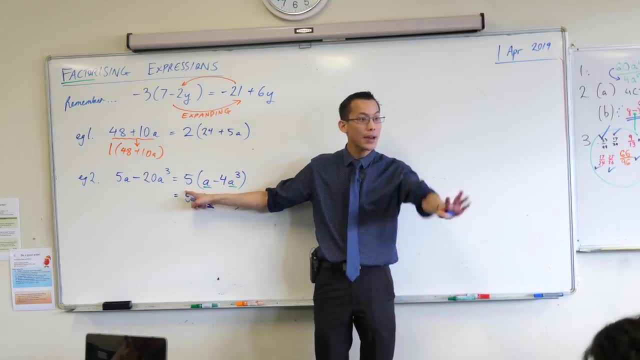 So you can see what we've done right. We took out the 5, and then we're like: wait, wait, wait, I can keep going. I can take out A as well. What do you think of this? Can we go any further? 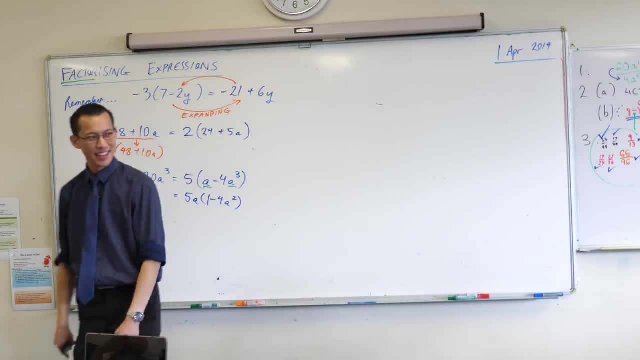 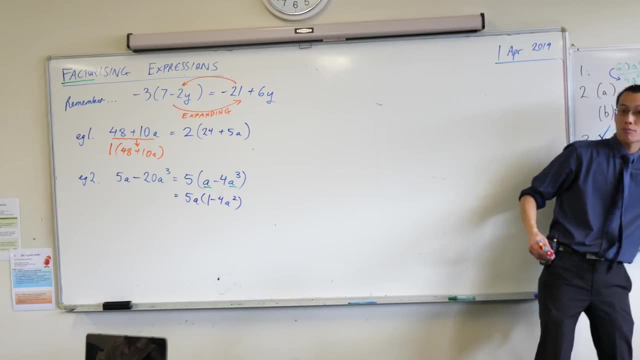 No, Hmm, Yes. So here's one of the cool things, right, Just put your pens down for a minute and look up When you were in, when you were in primary school, right? and someone said to you: can? 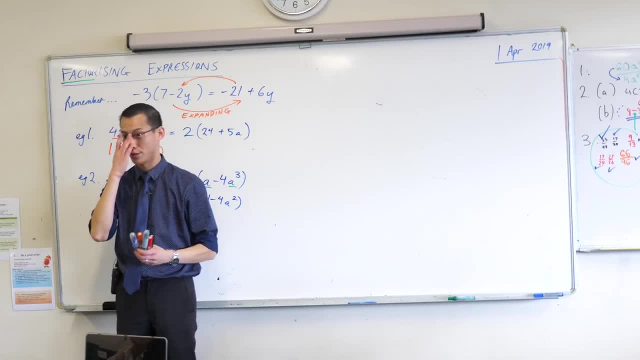 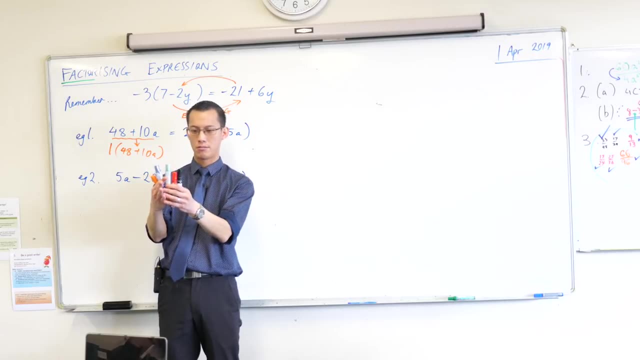 you and not a rhetorical question: can you tell me what 5 take away 3 is? You all would have said 2, right, Because 1,, 2,, 3,, 4,, 5, you can take away 3 objects: 1,, 2,, 3, and then you get left with 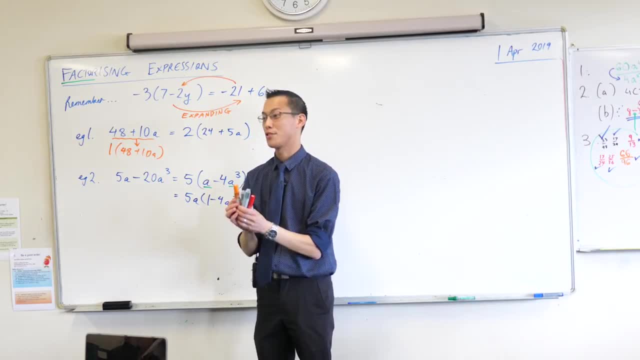 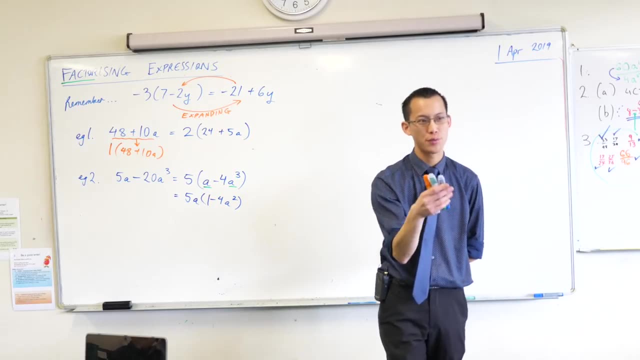 2, right And had someone asked you primary school. you, hey, can you do 3, take away 5? Primary school? you should have responded: you can't do that, because how can you take 5 away from this right? 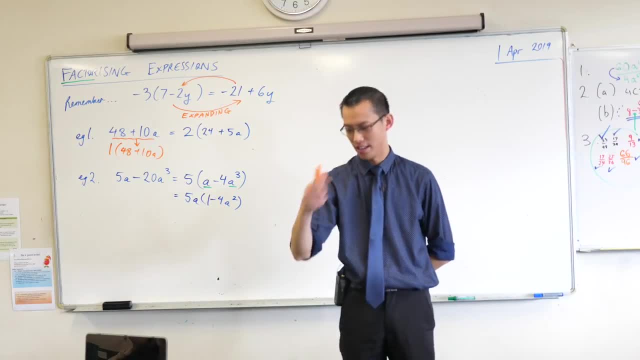 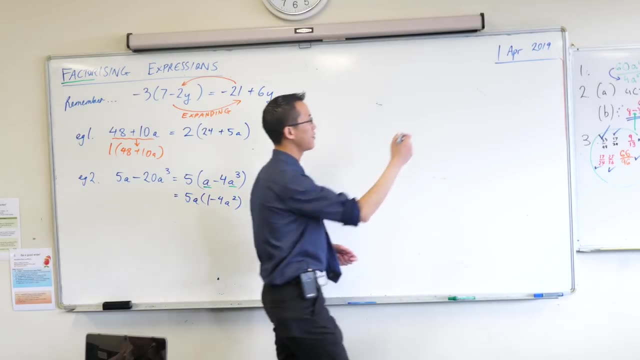 You're like: well, you take away 1, and then you take 2, and then you take away 3, and then I've got no more stuff to take away, right? But high school you knows that 3 take away 5 can be done right. 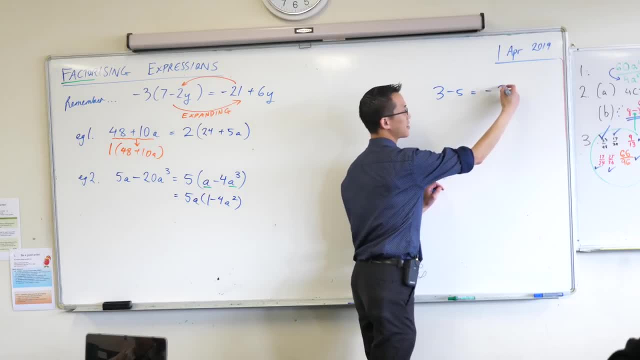 You can say: oh, I know what negative numbers are, So you have an answer for this, right? Do you agree with that? And what happens is the more that you know, the wider kind of problem you're going to solve, the wider kind of problems you can solve. 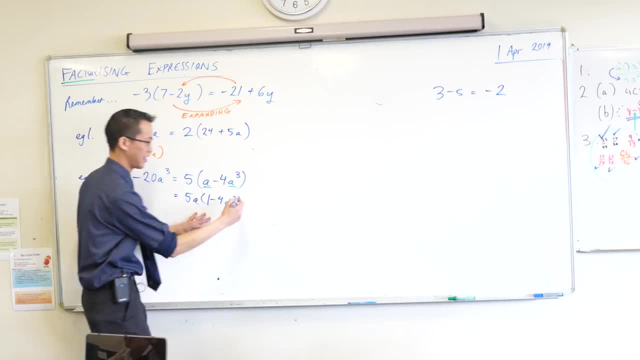 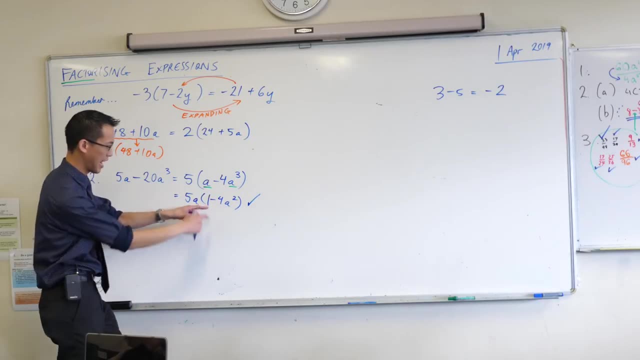 Now, at the moment, this is totally fine. Give it a big tick, okay, This is perfect, right. But as you go forward, you're actually going to learn how to. you can factorize this as well. You can take a common factor out. 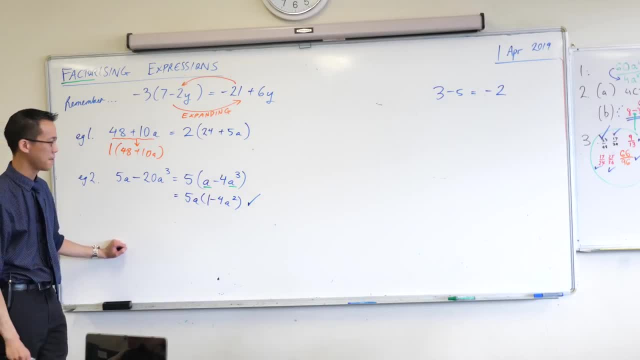 I'm going to teach you how to do that a little bit later on, okay, But for now, that's where we can stop. all right, Can you write down example 3 for me Now? this is when we're going to get to Krishan's question, because he was talking about negatives. 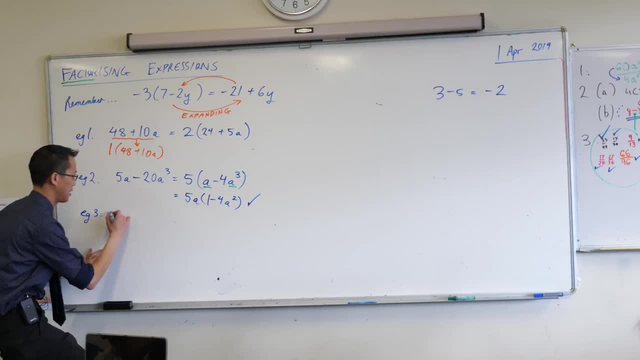 right, At least we're going to start to answer it. So here's what I'd like you to put down. What am I going to give you? I'm going to give you this. Actually, I'm going to. yeah, that'll do. 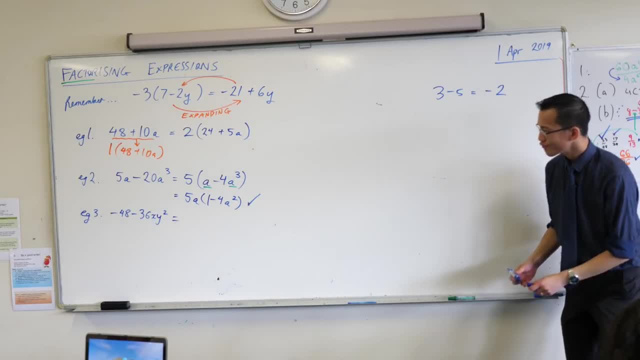 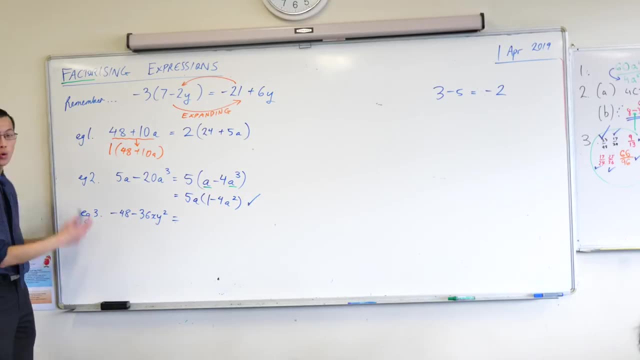 Okay, So this is starting to look a little messier, isn't it? Now, when you have a look at this, right, I'm going to ask the same question that I've been asking all the way through, And you might notice. you know, it's nice. 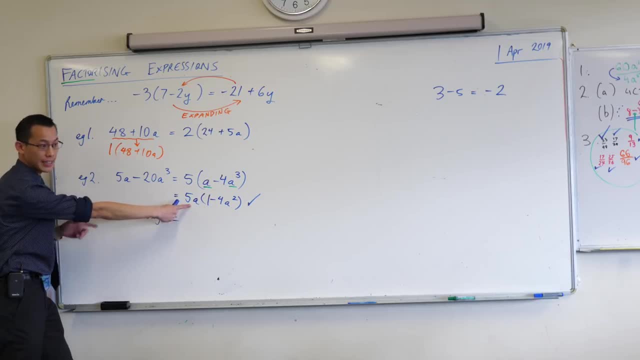 If you can look at this And you can say, oh, I can get 5A immediately, then go there. You don't have to do it in two steps, But often it takes some time to like recognize what are the things you can take out. 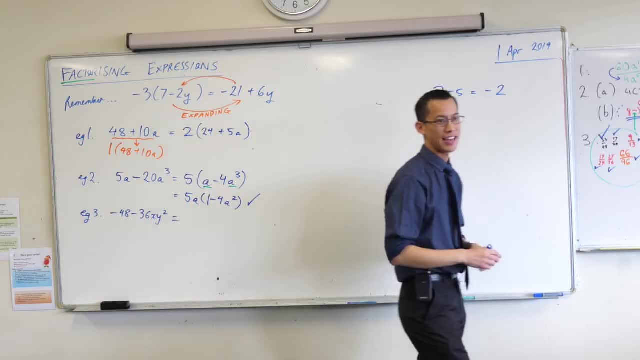 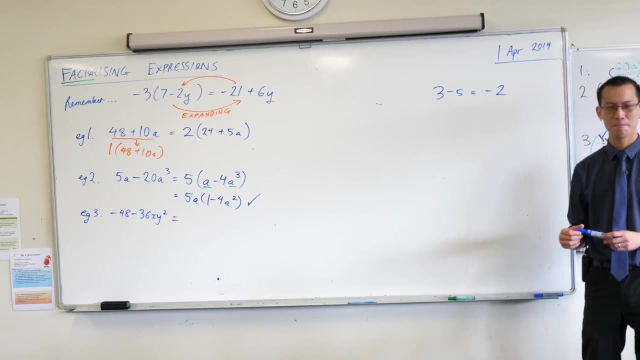 So can someone name for me just a single thing that they can take out? Okay, Jessica, why don't you hold that thought? You give me a few answers, which is great. Who else can give me a suggestion? Hmm, Tim, what do you see? 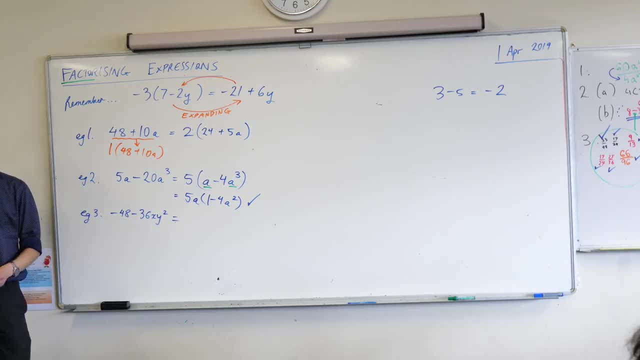 Tim, why don't you have a look? Example 3. Have a look at the numbers. Have a look at the pronumerals. Can you pick a number out, Any number that's a common factor between these two? Hmm, David, can you help him out? 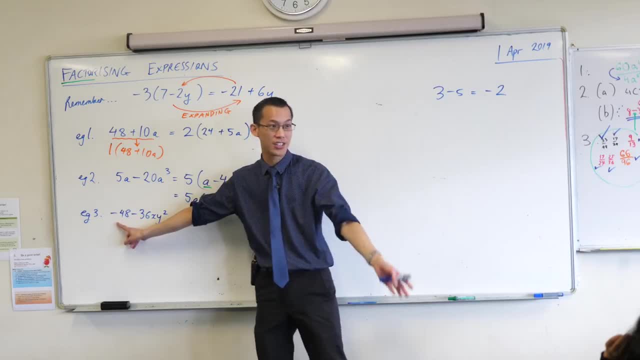 Can you see a number that you can divide into this? and you can divide into this as well Any number you like, Probably 4.. 4 works for me. Let's start with that. Okay, you might be able to think of another one. 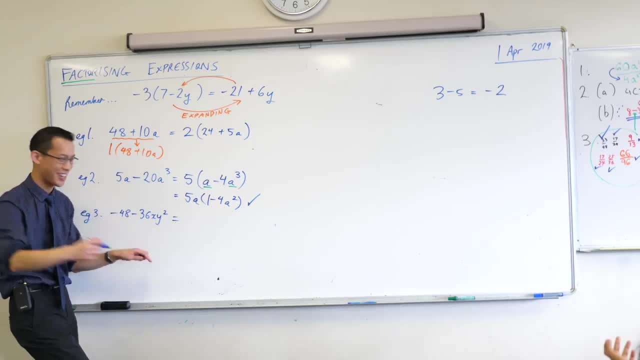 We'll come to you in a minute. Let's divide by 4.. Okay, and we'll get more suggestions in a second. Let's do 4 first. Okay, 4 was the suggestion. I want to honor that, Okay. 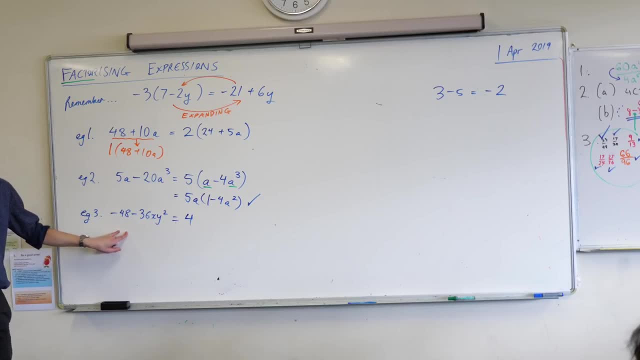 When you divide negative 48 by 4,, what do you get? 12.. Just watch out: You've got negative 48, right? So you're going to get negative 12.. Okay, Now I'm going to do the next one. 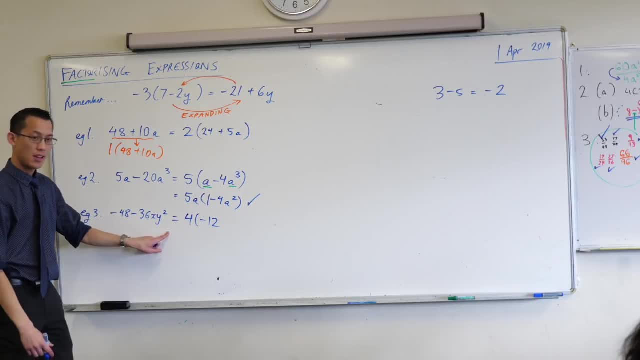 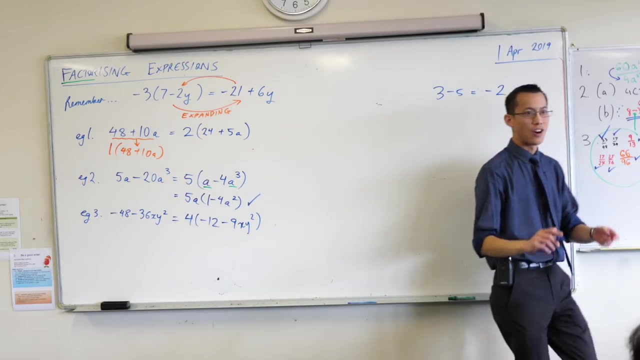 Negative, 36xy squared, That'll be minus. I'm dividing this by 4, aren't I? So I should get 9.. What happens to the pronumerals xy- xy squared? Nothing's changed. Okay Now, some of you had your hands up even after David suggested his number, because you're. 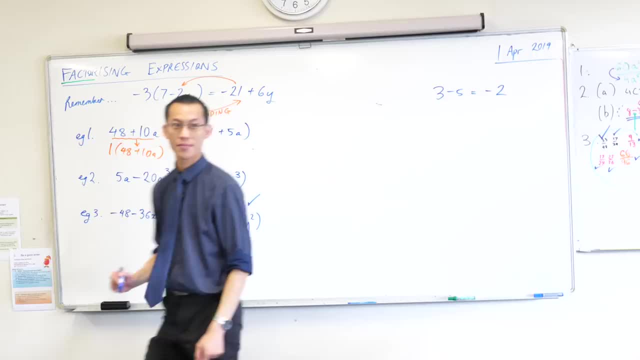 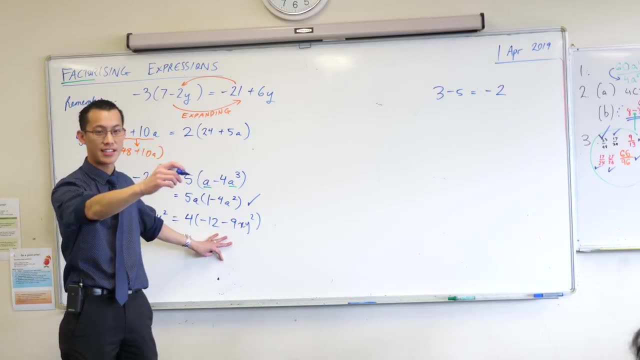 like: oh, I can do more. Right, Harry, what did you see? 12. I can see 12.. Now I can take 12 out from here, but at the moment, over here, having done David's suggested step, Jessica, having done David's suggested step, I can't divide these guys. 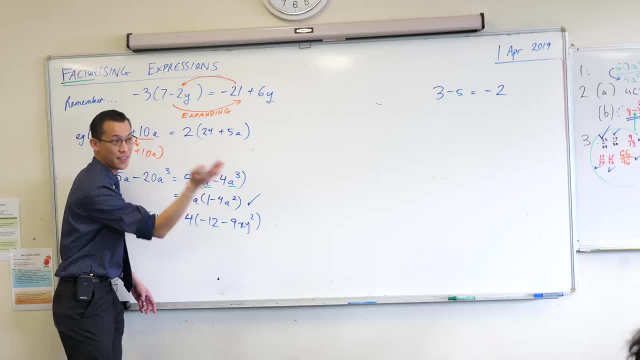 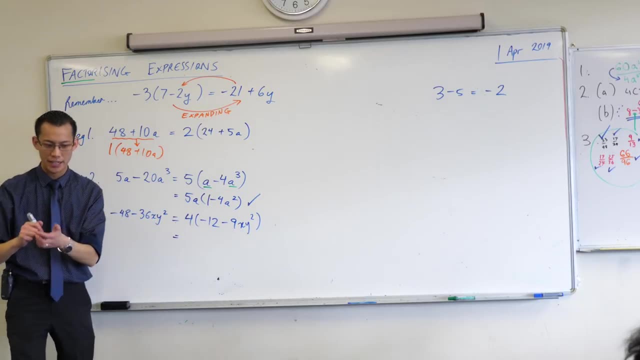 by 12 anymore, right? This one's too small. So what can I do instead? Vishakha 3.. I can do 3, right, 3 will go into 12 and it'll go into 9.. So when I'm put your pens down for a second, 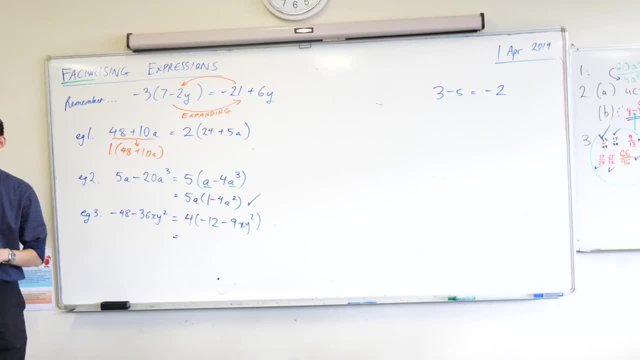 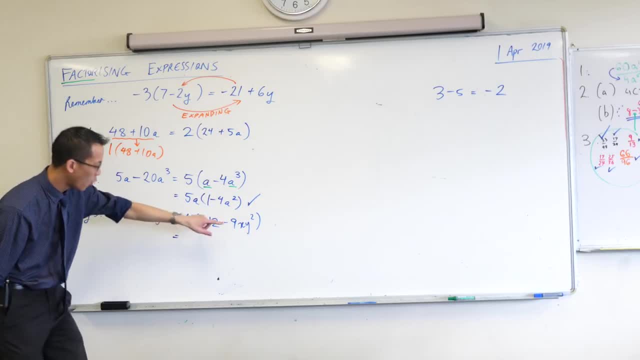 Now I've already got a 4 and Vishakha's suggesting that I also take out a 3.. So instead of having 4 out the front, I'm going to have the 4 and the 3 together. So that gives me 12, which is actually that number that Harry suggested in the first place. 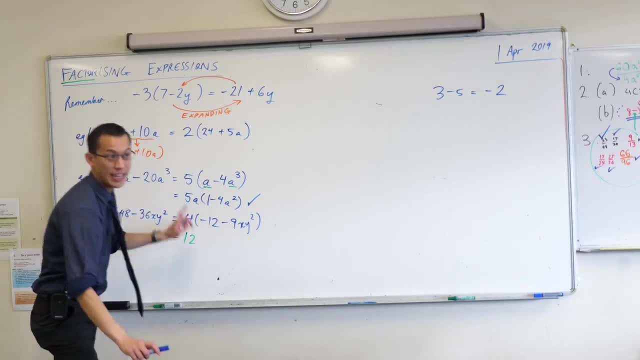 Okay. So can you highlight that for me? Because once you've already taken out one number, when you take out another one, the sort of collect at the front- Okay, All right, Now we're taking out 3.. What will happen with this minus 12?? 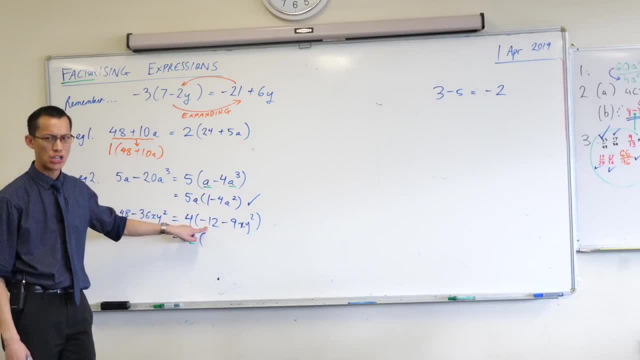 When you divide it by 3? Yeah here, Negative 4.. Negative 4.. Thank you very much. I'm going to divide this by 3 as well. What are you going to get? Vishakha 3 x minus 12.. 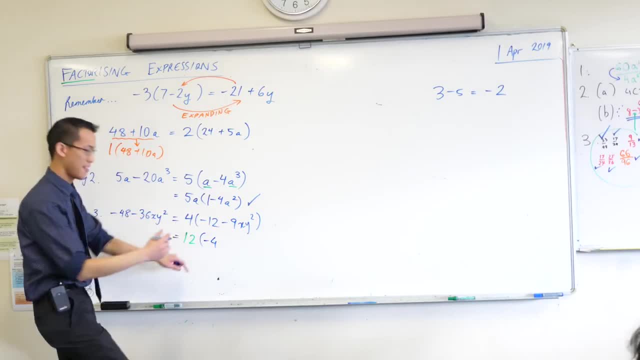 Very good. Okay, Now at this point, the pronumerals. there's nothing much that we can do with those pronumerals. The numbers look pretty good. 4 and 3 are very small. Right, But there's one more thing we can do which will be interesting. 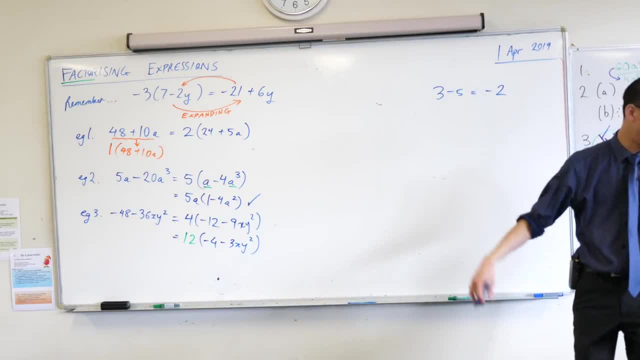 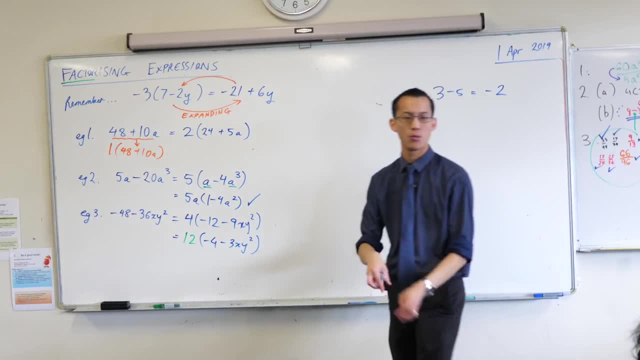 Right, And I'm like: I don't like negatives, They're gross. I want to write as few negatives as I can, because negatives are easy to confuse, So I'm going to do one last thing. I'm going to take out negative 1.. 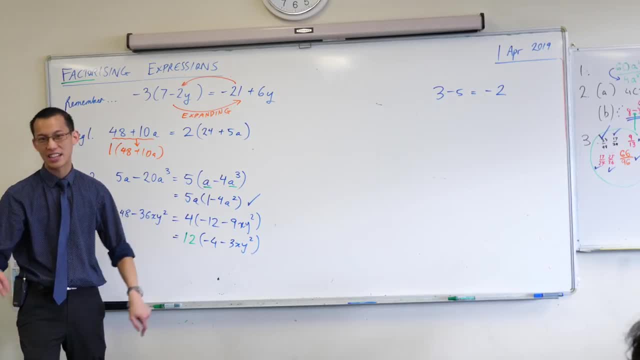 Yes, I knew it. Okay, Yay, Right, And they picked it Right. It's like that feeling of I knew that was the bad guy, Okay, So if I take out a minus sign, I'm going to get negative 1.. 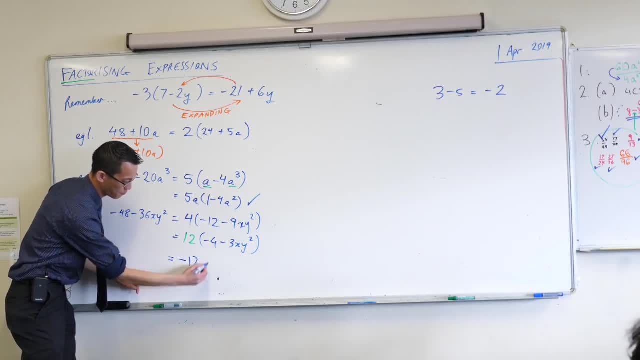 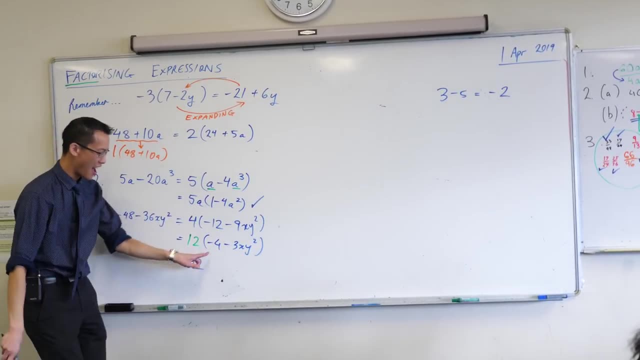 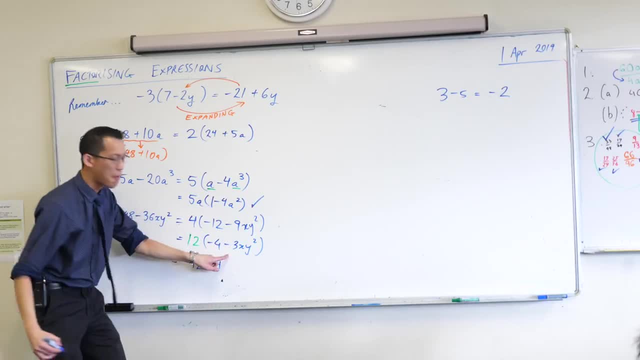 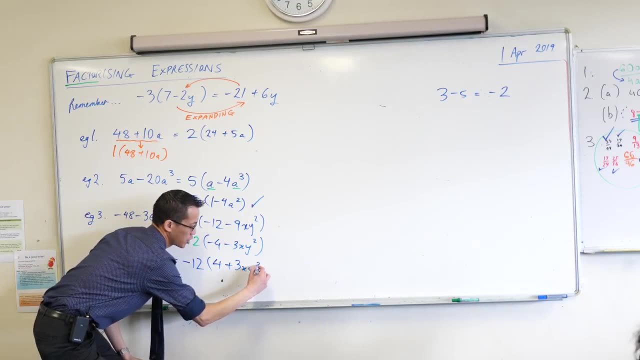 It'll be Positive 4. Positive 4. Right, Just regular old 4.. This minus 3 x, y squared, will not be minus anymore, It'll be Positive, Positive, Plus. Now, just before I show you, or actually let you loose on some of the textbook exercises: 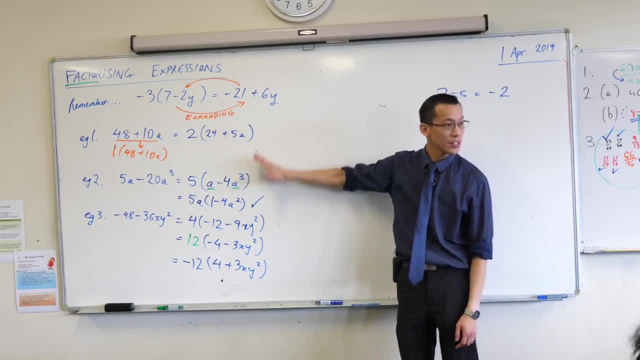 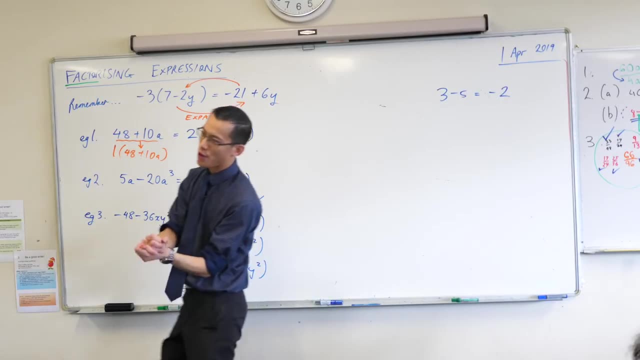 one of the great things about all of these questions is: Have a look at example one, two and three. Your final line is: this factorized thing, This factorized thing. You can always know whether your factorization is right by checking it really simply.